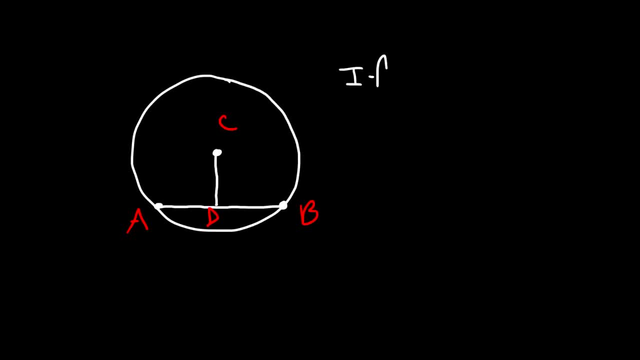 Now if segment C, D is perpendicular to AB, so if we draw in such a way that C, D and AB meet at a right angle, then C? D bisects AB. So that means that AD And D- B are congruent. 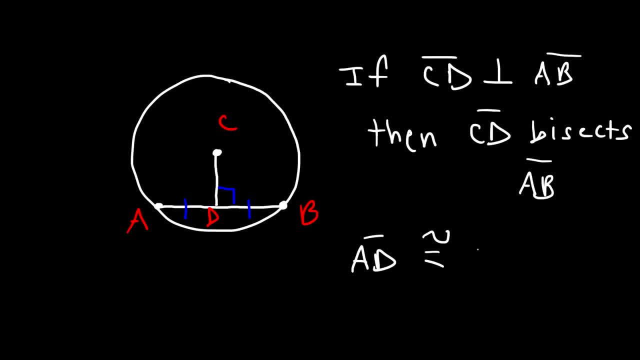 So make sure you understand that. So if you draw a segment between the center of a circle to any chord, and if you draw it at a right angle, then this segment becomes the perpendicular bisector of the chord. So AD is congruent to D, B. 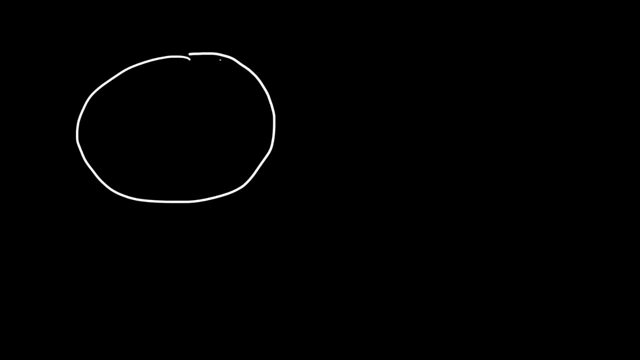 Now there's another theorem that you need to know about chords. So let's say this: This is the center, and we have a chord here and another chord here. Let's call this chord AB and DE, And this is going to be center C. 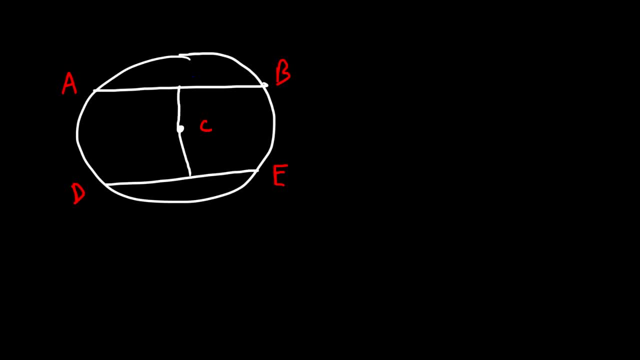 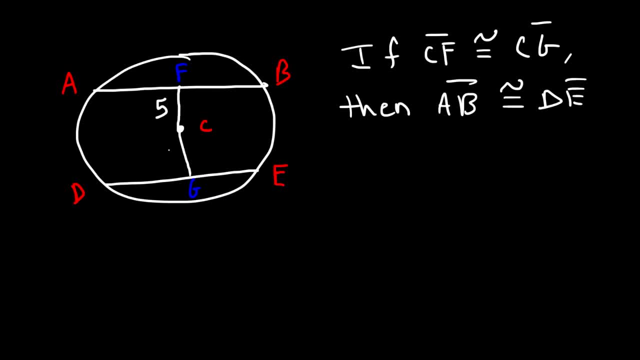 So let's say, if CF is 5, and CG is 5.. Now, if AB is equal to 12,, what is the value of DE? So, if these two are congruent, if they're equal to each other, and that means that DE is going to be equal to AB, 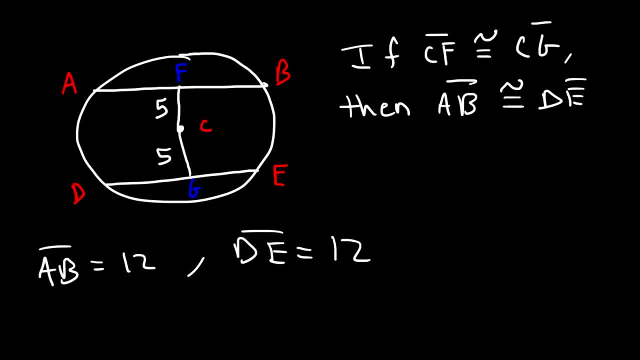 So if AB is 12, DE is 12.. So that's the concept of congruent chords: If they're equidistant from the center, then they are congruent. So anytime two chords of a circle are equidistant from the center, 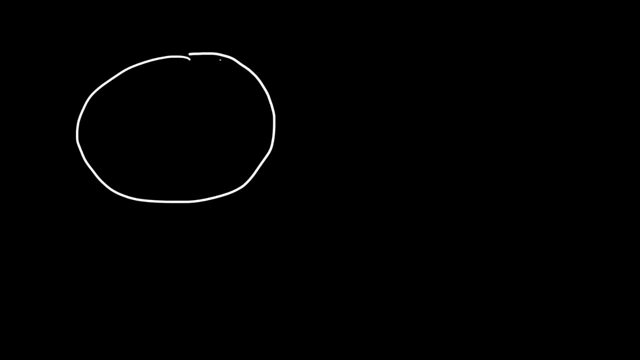 Now there's another theorem that you need to know about chords. So let's say this: This is the center, and we have a chord here and another chord here. Let's call this chord AB and DE, And this is going to be center C. 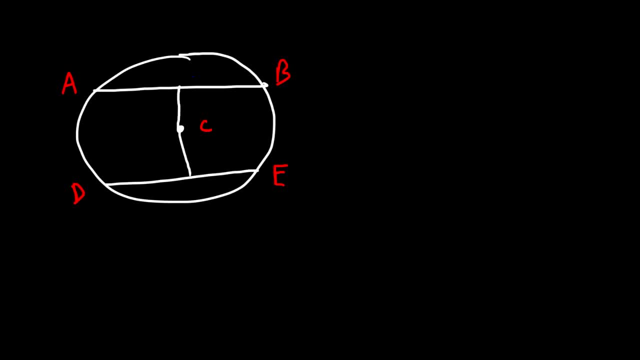 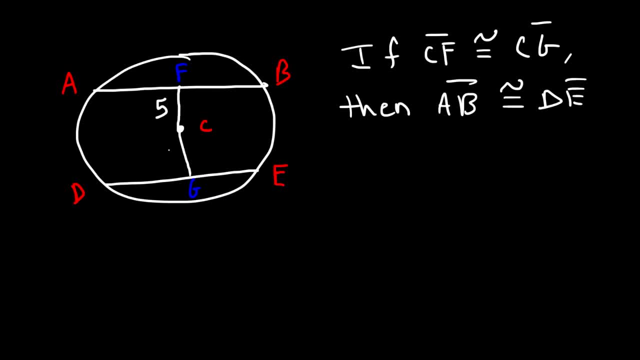 So let's say, if CF is 5, and CG is 5.. Now, if AB is equal to 12,, what is the value of DE? So, if these two are congruent, if they're equal to each other, and that means that DE is going to be equal to AB, 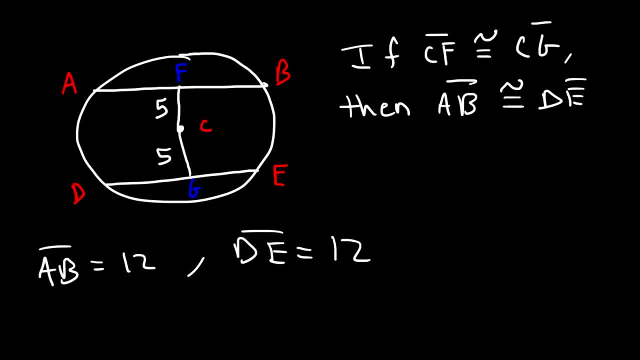 So if AB is 12, DE is 12.. So that's the concept of congruent chords: If they're equidistant from the center, then they are congruent. So anytime two chords of a circle are equidistant from the center, 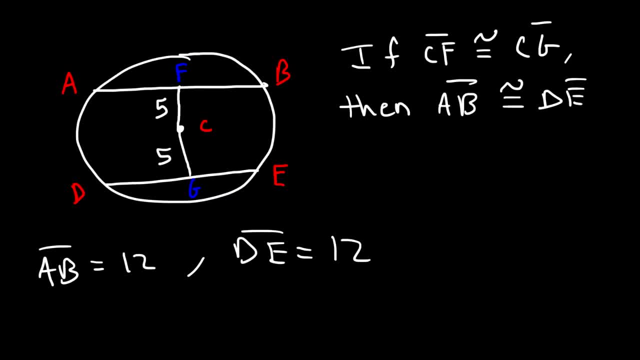 then the two chords are congruent. Now, what if CF is perpendicular to AB? What do we know from the last theorem? If that's the case, then F is the midpoint of AB. So AF is congruent to FB. And if CG is perpendicular to DE, that means that DG has to equal GE. 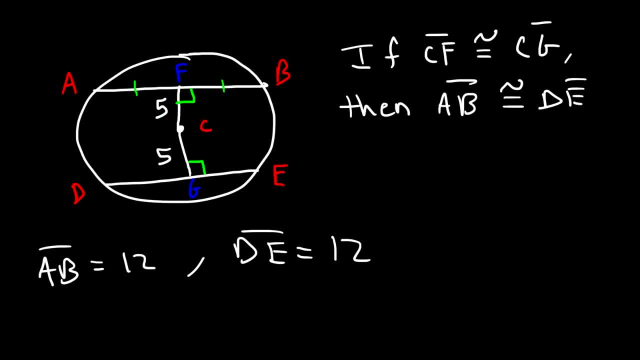 And if these two are equal to 12, then these sides will not only be equal to each other, but they're also equal to the other sides as well. So those are some theorems to keep in mind when you're dealing with chords and circles. 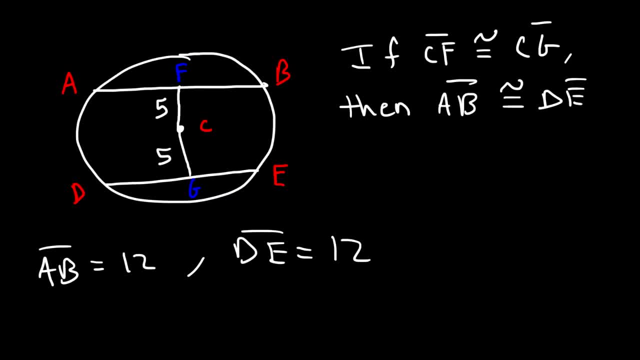 then the two chords are congruent. Now, what if CF is perpendicular to AB? What do we know from the last theorem? If that's the case, then F is the midpoint of AB. So AF is congruent to FB. And if CG is perpendicular to DE, that means that DG has to equal GE. 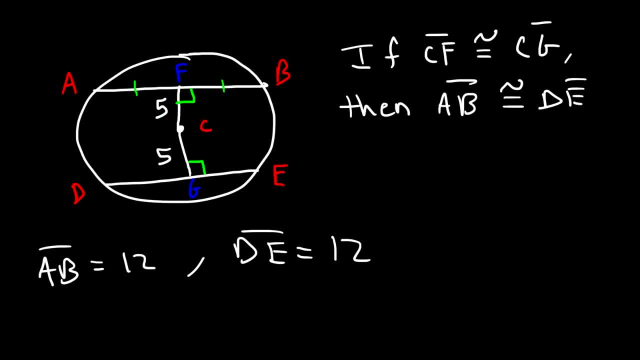 And if these two are equal to 12, then these sides will not only be equal to each other, but they're also equal to the other sides as well. So those are some theorems to keep in mind when you're dealing with chords and circles. 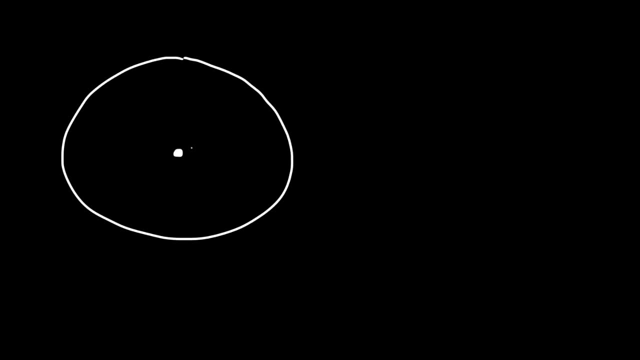 Now let's work on some problems. So let's say this is the center and we have a chord here and another chord there. Let's call this chord AB and DE, And this is going to be center C. Let's call this point F and G. 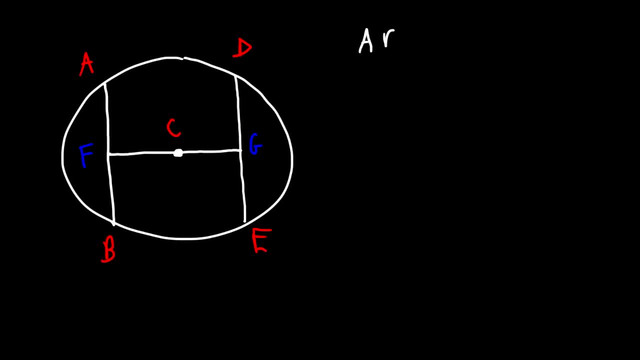 So let's say that you're given AB is equal to DE, And let's say that CF is equal to 5X plus 3.. And CG is equal to 7X minus 5.. So, with this information, what is the length of, let's say, FG? 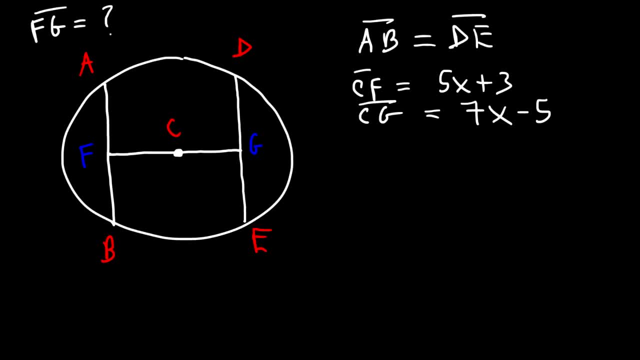 Feel free to pause the video. So first we need to calculate the value of X. If AB is equal to DE, then we know that CF and CG are equal to each other. So let's set them equal to each other. So that means that 5X plus 3 has to equal 7X minus 5.. 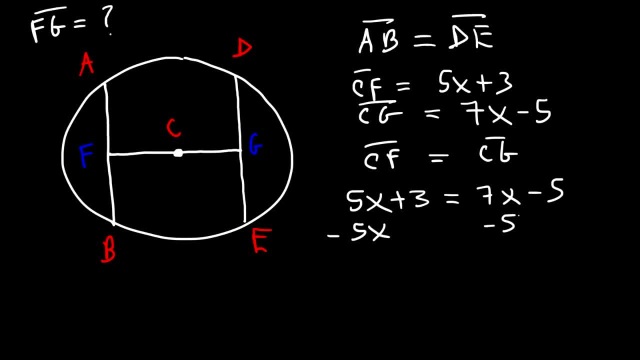 So let's subtract both sides by 5X And let's add 5 to both sides, So we can cross out these two: 3 plus 5 is 8. And 7X minus 5X is 2X. 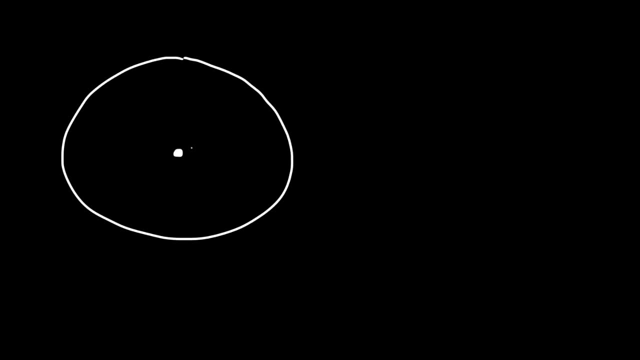 Now let's work on some problems. So let's say this is the center and we have a chord here and another chord there. Let's call this chord AB and DE, And this is going to be center C. Let's call this point F and G. 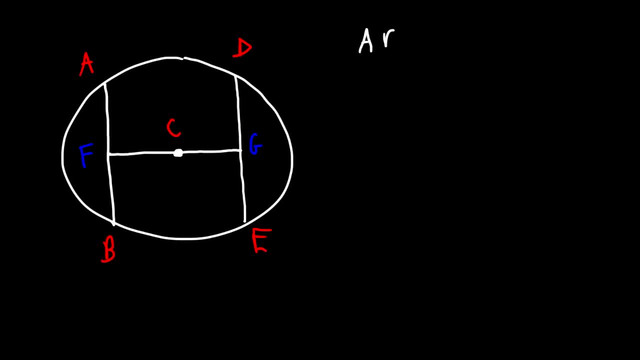 So let's say that you're given AB is equal to DE, And let's say that CF is equal to 5X plus 3.. And CG is equal to 7X minus 5.. So, with this information, what is the length of, let's say, FG? 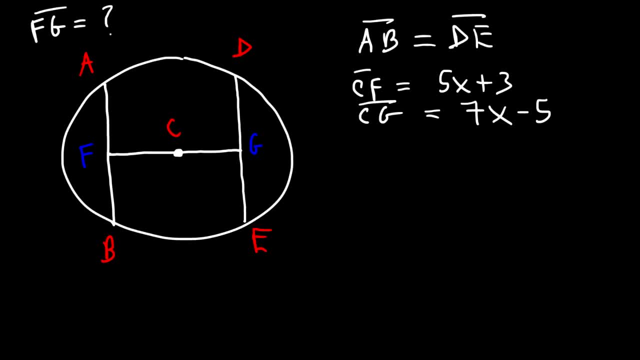 Feel free to pause the video. So first we need to calculate the value of X. If AB is equal to DE, then we know that CF and CG are equal to each other. So let's set them equal to each other. So that means that 5X plus 3 has to equal 7X minus 5.. 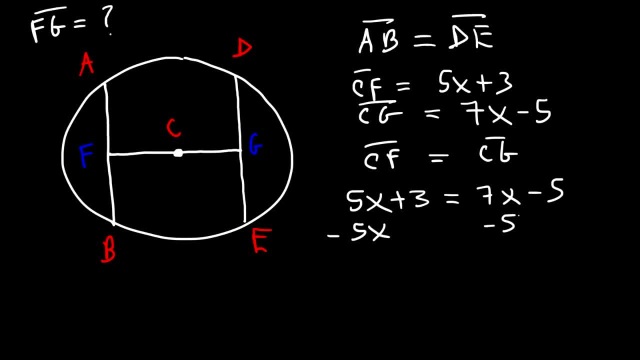 So let's subtract both sides by 5X And let's add 5 to both sides, So we can cross out these two: 3 plus 5 is 8. And 7X minus 5X is 2X. 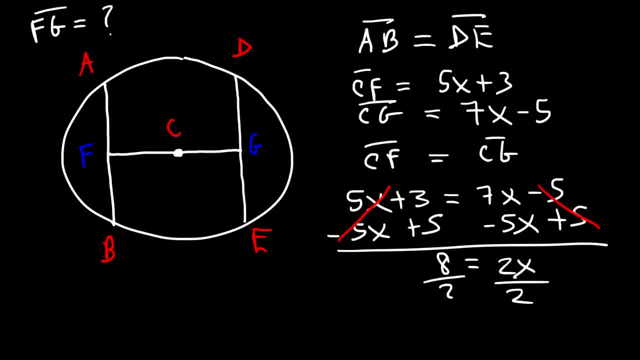 Now let's divide both sides by 2.. So 8 divided by 2 is 4.. So X is equal to 4.. So now we can find the value of CF. So that's 5 times 4 plus 3.. 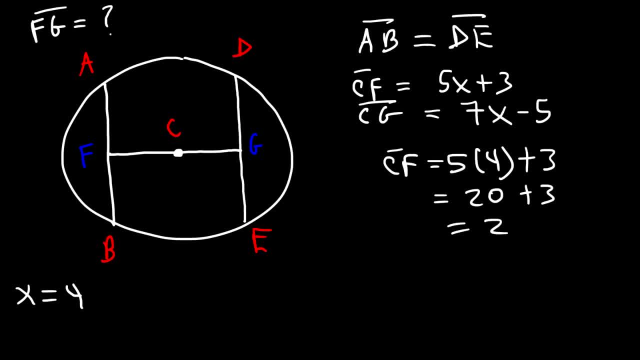 5 times 4 is 20.. 20 plus 3 is 23. 23. Well, CF is 23.. Which means that CG is 23.. Now, FG is the sum of FC and CG, So it's 23 plus 23,, which is 46.. 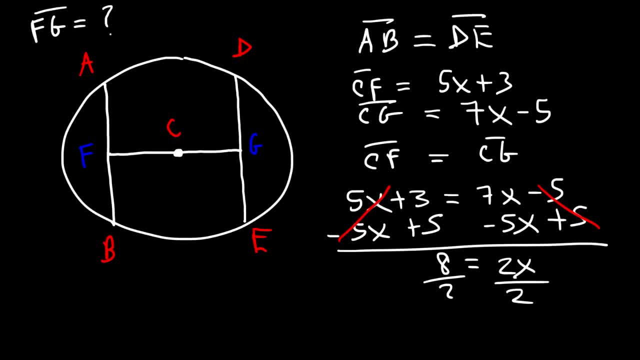 Now let's divide both sides by 2.. So 8 divided by 2 is 4.. So X is equal to 4.. So now we can find the value of CF. So that's 5 times 4 plus 3.. 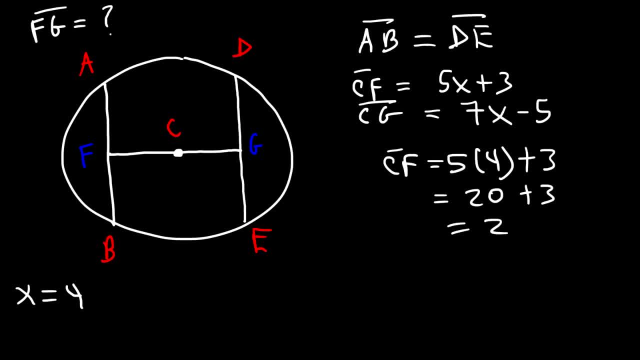 5 times 4 is 20.. 20 plus 3 is 23. 23. Well, CF is 23.. Which means that CG is 23.. Now, FG is the sum of FC and CG, So it's 23 plus 23,, which is 46.. 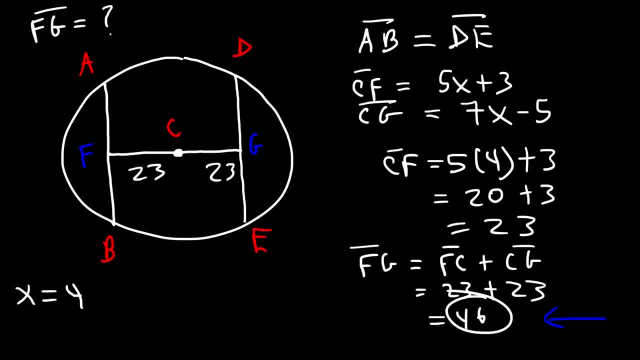 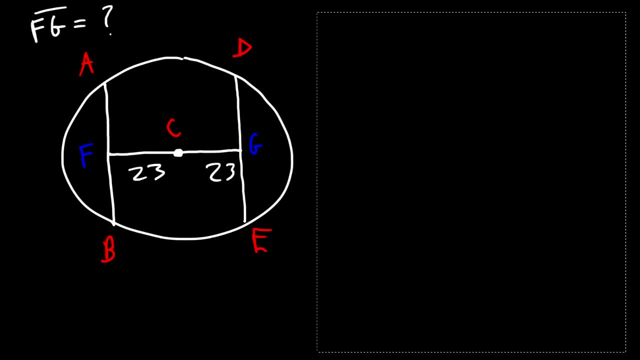 So this is the answer, And so that's it for this problem. Now I'm going to give you another problem that's related to this circle. Okay, Now let me get rid of this too. So let's say that CG is perpendicular to DE. 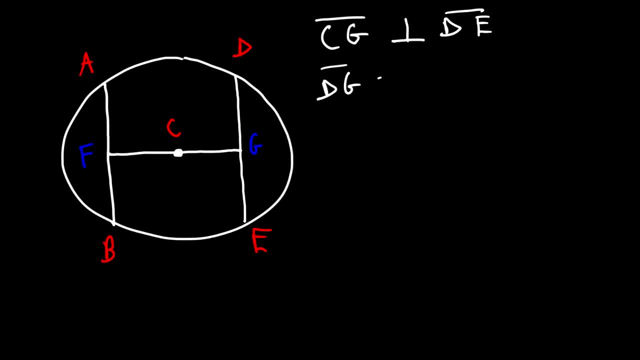 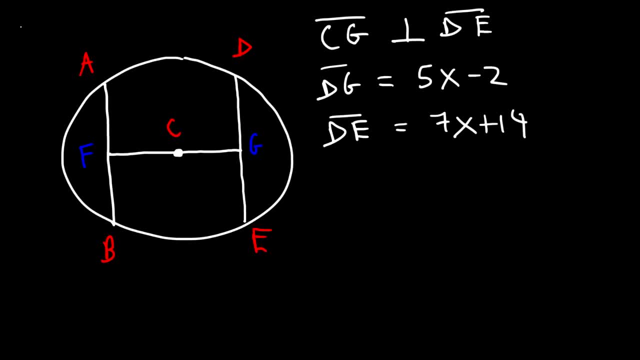 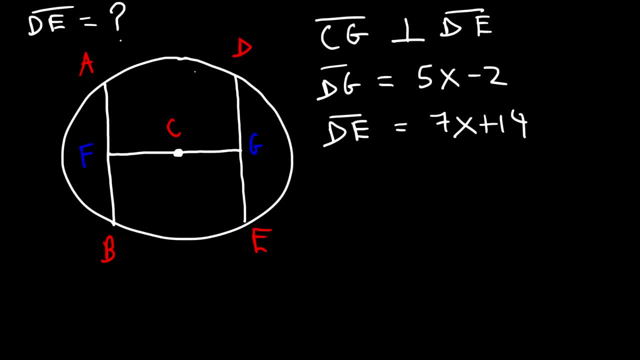 So feel free to pause the video if you want to try this problem. Now. if CG is perpendicular to DE, we know that DG and GE are congruent. So let's say, if DG is 5.. 7X plus 4.. 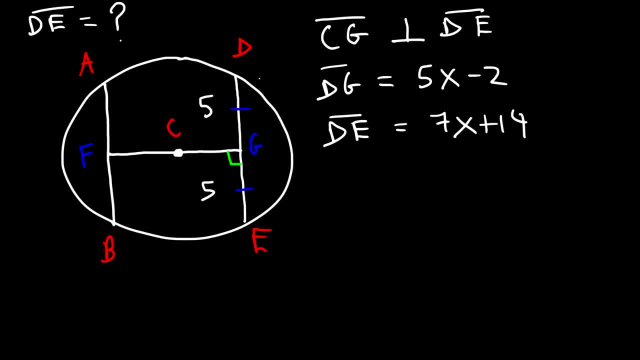 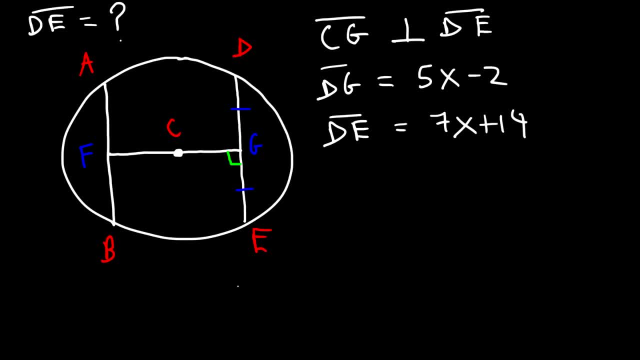 4X plus 4.. 3X plus 2.. 3X plus 7.. 7X plus 8. 7X plus 1. 3X plus 4., 4., 4., 14.. 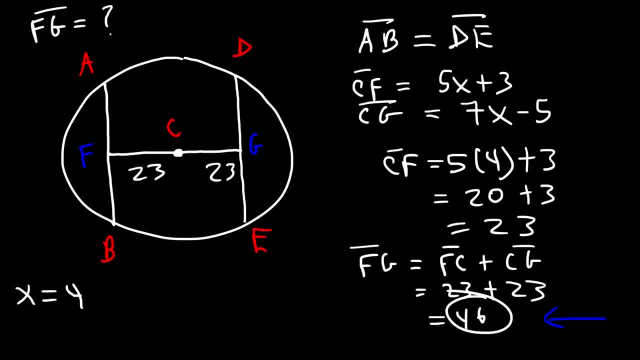 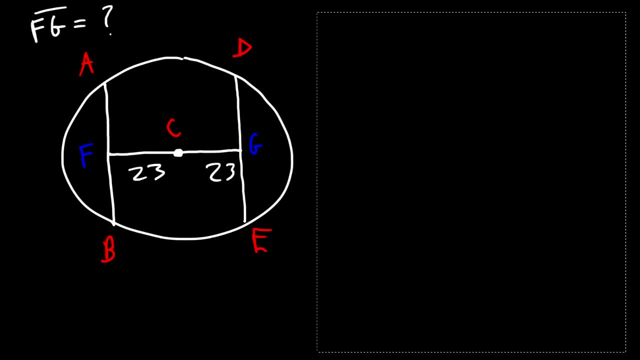 So this is the answer, And so that's it for this problem. Now I'm going to give you another problem that's related to this circle. Okay, Now let me get rid of this too. So let's say that CG is perpendicular to DE. 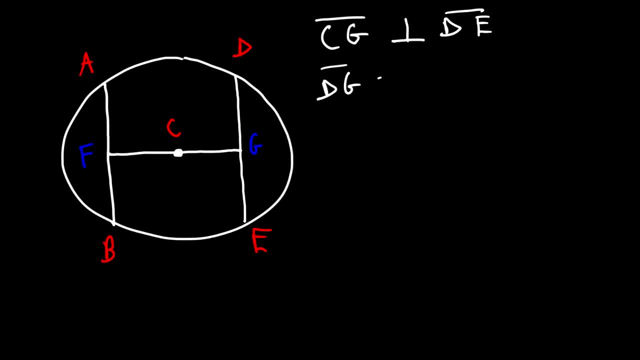 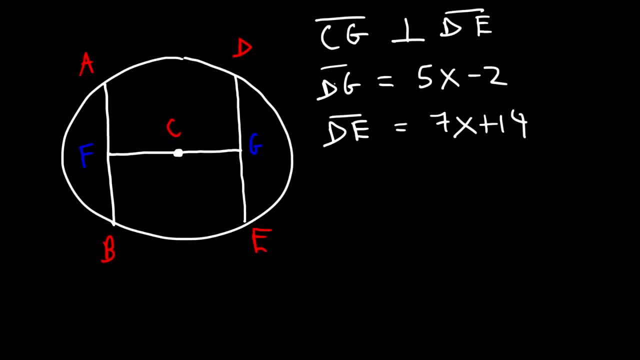 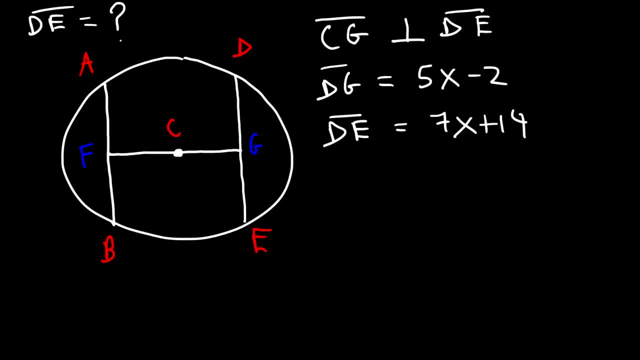 How long is it? So feel free to pause the video if you want to try this problem Now. if CG is perpendicular to DE, we know that DG and GE are congruent. So let's say, if DG is 5.. that means the GE is 5, but DE itself, the whole thing has to be 10 and 5 is half. 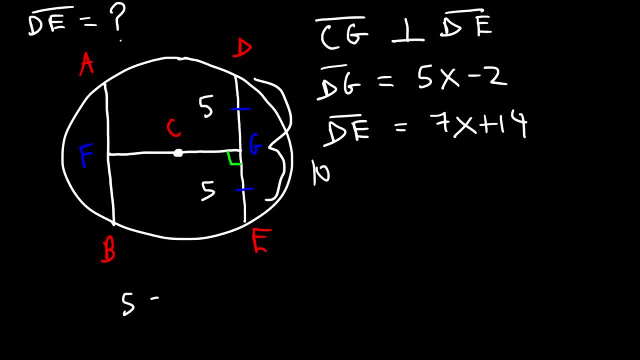 of 10. so therefore we could say that DG is one half of DE. so if DG is 5x minus 2, that has to be one half of 7x plus 14. now let's calculate the value of X. let's multiply both sides by 2, so half of 2 is 1, and 2 times 5x is 10x. we need to. 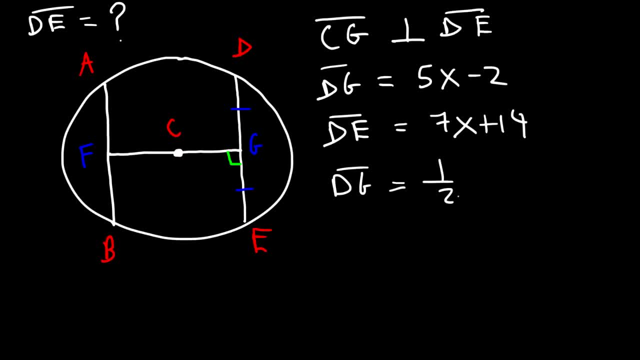 4. Dnes получилось 14. 5. 1.. 59. 0., 0., 0., 25.. 96., 13. 17. 1., 2., 2.. 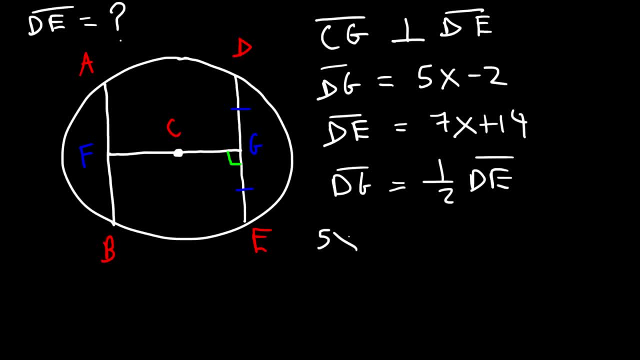 1. 0., 2., 9., 5., 7., 73., 3., 90., 8., 30., 22. 35.. one half of 7x plus 14.. Now let's calculate the value of x. Let's multiply both sides by 2.. So 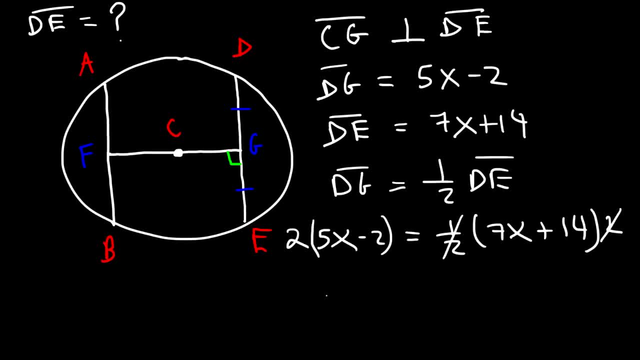 half of 2 is 1. And 2 times 5x is 10x. We need to distribute. And then 2 times negative 2 is negative 4.. And once we get rid of the one half on this side, we don't need the parentheses. So 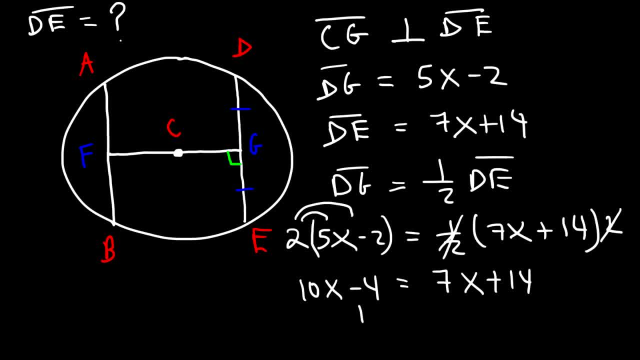 it's just 7x plus 14.. So now let's add 4 to both sides And let's subtract both sides by 7x. So 10x minus 7x is 3x, And 14 plus 4 is 18.. So now let's divide both sides by 3.. 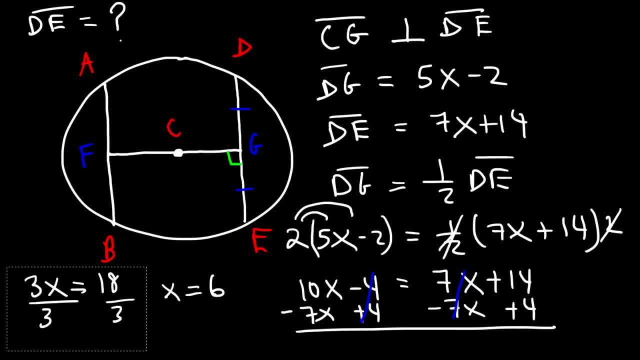 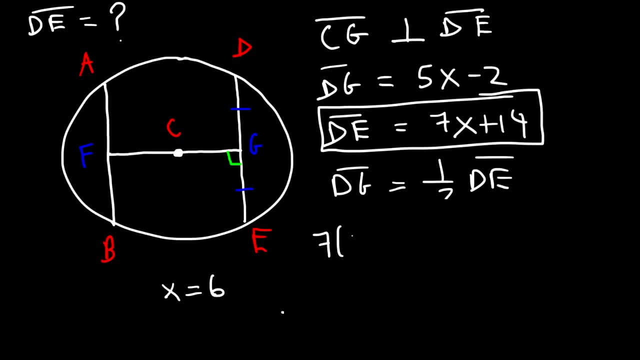 18 divided by 3 is 6.. So x is equal to 6.. So now we can calculate dE using this expression. So 7 times 6 plus 14.. 7 times 6 is 42.. 42 plus 14. 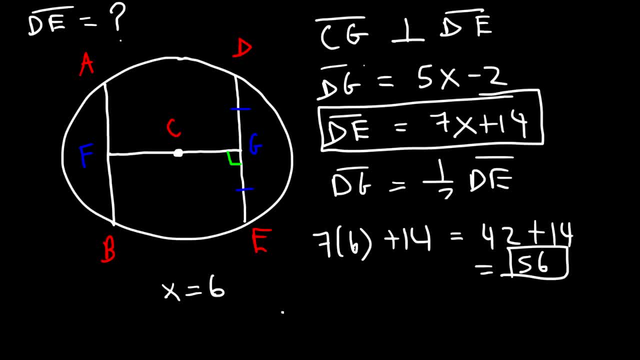 is 56. And we know that dG is half of dE, So dG is 28.. gE is 28. But dE as a total like the whole thing of 56, and so that's the answer for this problem. now let's work on some word. 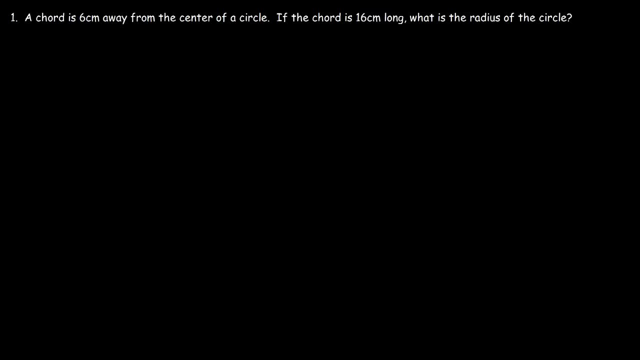 problems. a cord is 6 centimeters away from the center of a circle. if the cord is 16 centimeters long, what is the radius of the circle? so let's start with a picture and let's say this is the center and let's say this is the cord. 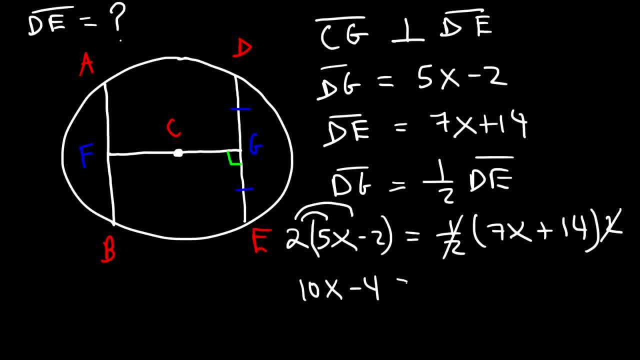 distribute and then 2 times negative. 2 is negative 4, and once we get rid of the one half on this side, we don't need the parentheses, so it's just 7x plus 14. so now let's add 4 to both sides and let's subtract both sides by 7x. so 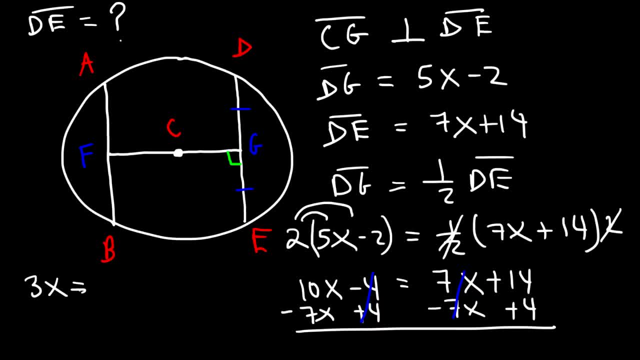 10x minus 7x is 3x, and 14 plus 4 is 18. so now let's divide both sides by 3: 18 divided by 3 is 6, so X is equal to 6. so now we can calculate DE using this expression. so 7 times 6 plus 14, 7 times. 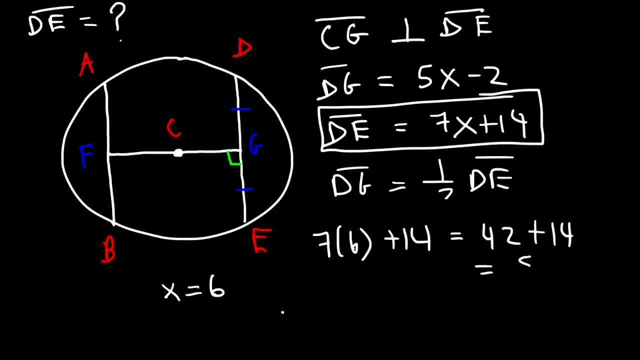 6 is 42, 42 plus 14 is 56, and we know that DG is half of DE. so DG is 28, GE is 28, but DE as a total, like the whole thing, that's a 56, and so that's the answer for this problem. now let's work on some word. 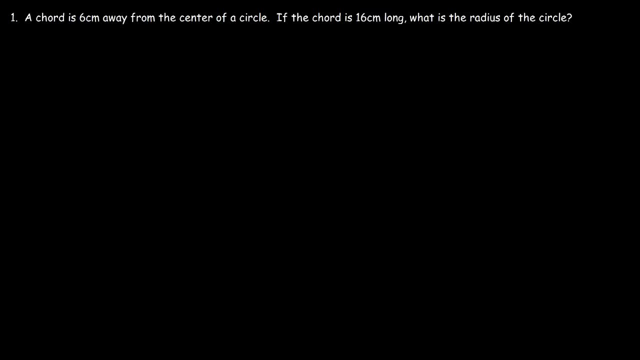 problems. a chord is 6 centimeters away from the center of a circle. if the chord is 16 centimeters long, what is the radius of the circle? so let's start with a picture and let's say this is the center and let's say this is the chord. 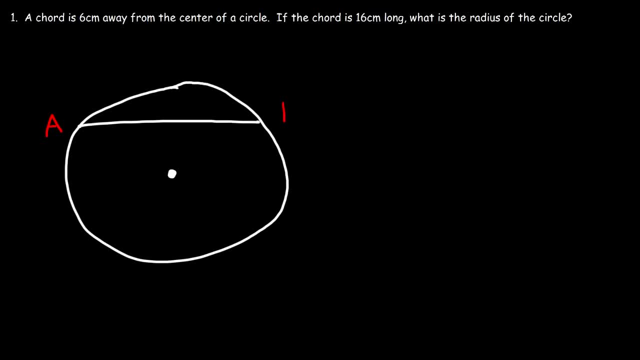 let's call it chord 8 b. this is center C. we'll call this point D, so let's draw a perpendicular line between the center and segment a be that's going to be the shortest distance between the center and the chord, and so these two are meet at right angles now. 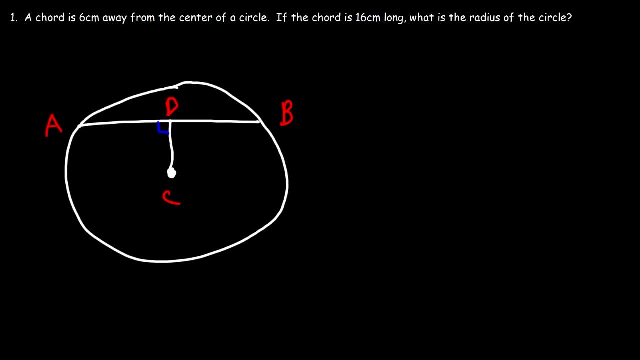 we know that the chord is six centimeters away from the center of the circle. so that means CD is six units long. now the cord is 16 centimeters, so segment AB is 16 minutes long and we know that if CD is perpendicular to AB, then AD and DB. 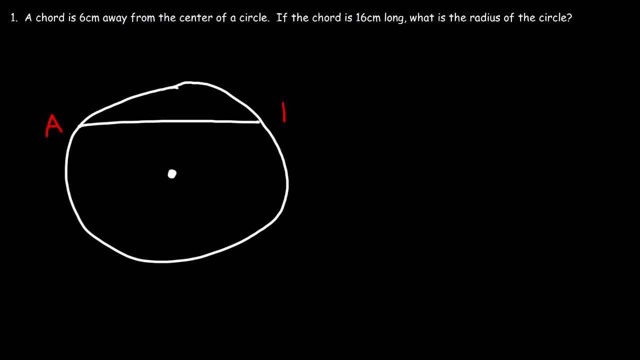 let's call it cord a B. this is center C, and we'll call this point D. so let's draw a perpendicular line between the center and segment a B. that's going to be the shortest distance between the center and the cord, and so these two will meet at right angles. now we know that the cord is 6 centimeters. 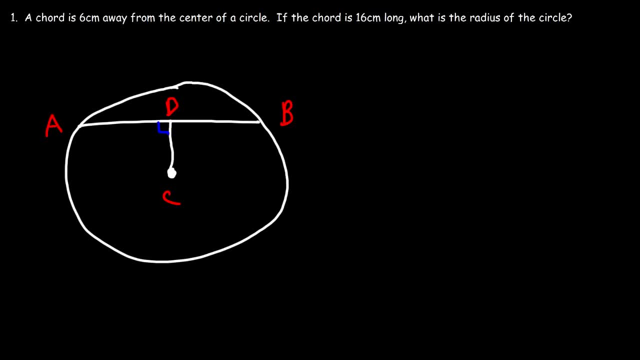 away from the center of the circle. so that means cd is 6 units long. now the cord is 16 centimeters, so segment a- b is 16 minutes long. and we know that if cd is perpendicular to a B then a, D and DB are congruent. so DB has to be half of a B. 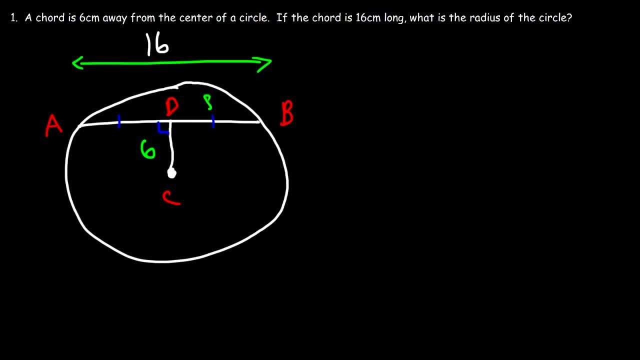 half of 16 is 8, so let's work on that. Let's put an 8 here. Now, the radius is the distance from the center of the circle to any point on the circle. So that's the radius of the circle. So basically, we need to calculate the hypotenuse of the right triangle. 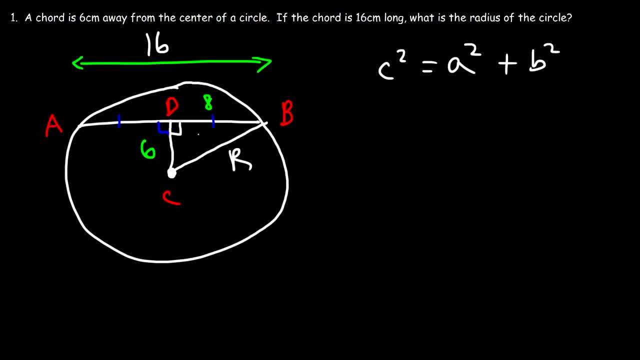 So we could use the Pythagorean theorem. So the hypotenuse is the radius of the circle, so that's r. Let's say that a is 6 and b is 8.. 8 squared is 36,, 8 squared is 64.. 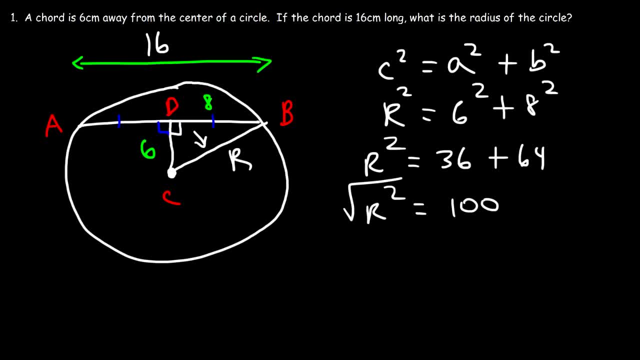 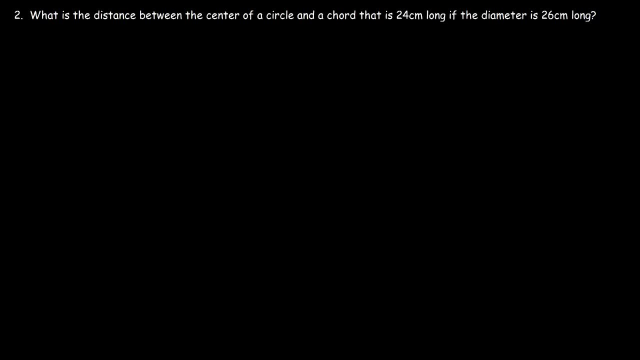 36 plus 64 is 100.. So if we take the square root of both sides, we could see that the radius of the circle is 10 units long, or 10 centimeters long Number 2.. What is the distance between the center of a circle and a chord? that is 24 centimeters. 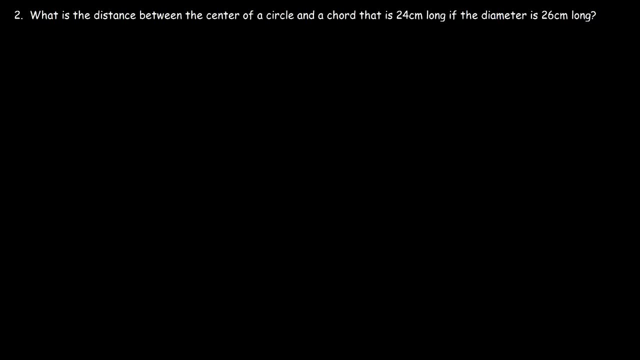 long if the diameter is 26 centimeters long. Okay, So go ahead and try this problem. Let's say this is the center and this is the chord of interest and this is going to be the diameter of the circle. So let's call this chord a, b, center c and point d. 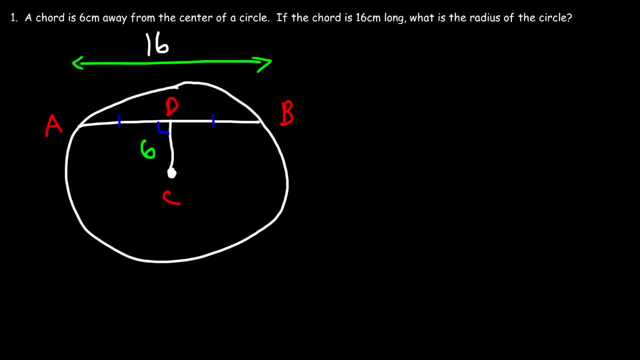 are congruent. so DB has to be half of AB. half of 16 is 8, so let's put an 8 here. now. the radius is distance from the center of the circle to any point on a circle. so that's the radius of the circle. so basically, we need to calculate. 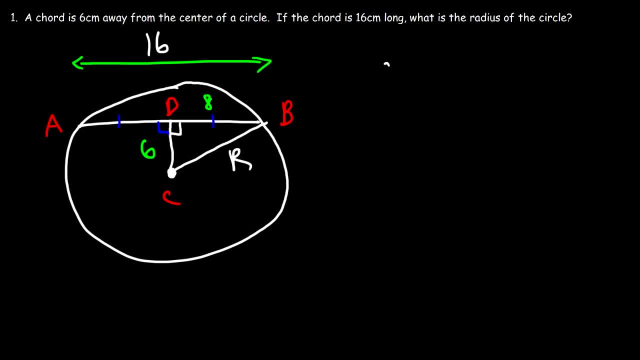 the hypotenuse of the right triangle. so we could use the Pythagorean theorem. so the hypotenuse is the radius of the circle. so that's R. let's say that A is 6 and B is 8. 6 squared is 36, 8 squared is 64. 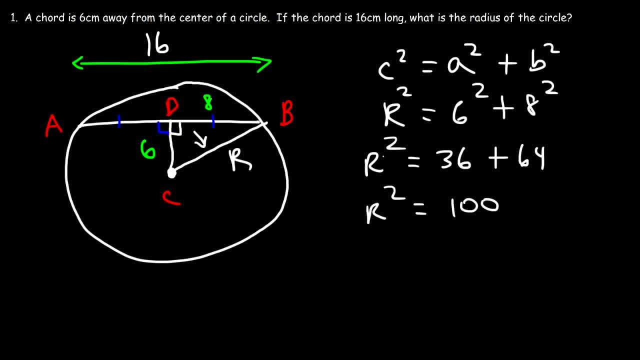 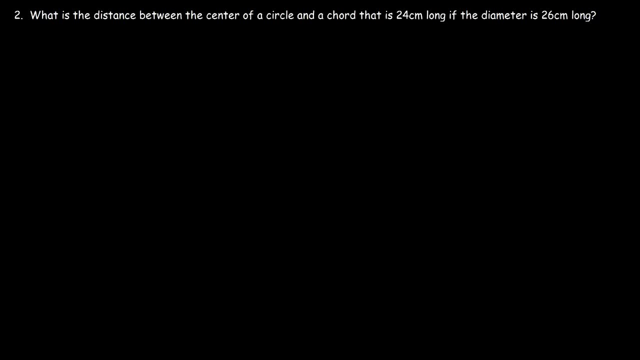 36 plus 64 is 100.. So if we take the square root of both sides, we could see that the radius of the circle is 10 units long or 10 centimeters long. Number two: what is the distance between the center of a circle and a chord? that is 24. 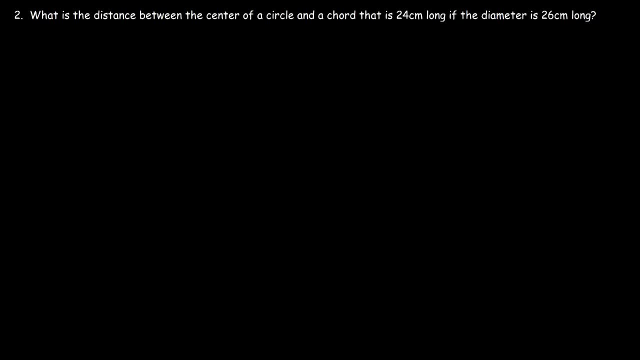 centimeters long if the diameter is 26 centimeters long. So go ahead and try this problem. Let's say this is the center and this is the chord of interest and this is going to be the diameter of the circle. So let's call this chord AB, center C and point D. So D is the midpoint of AB, as long. 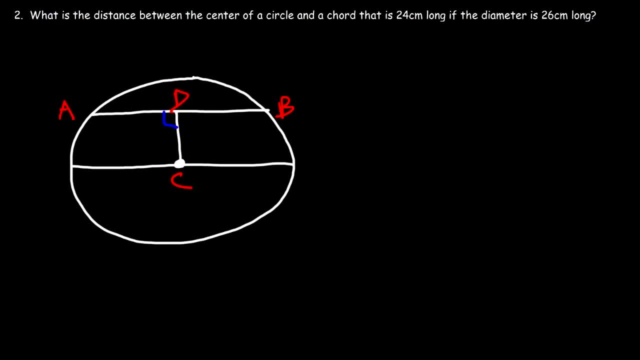 as CD is perpendicular to AB. Now we know that the chord is 24 centimeters long, So AB is 24.. And since CD is perpendicular to AB, AD is equal to DB. Those two segments are congruent, which means DB has to be 12.. 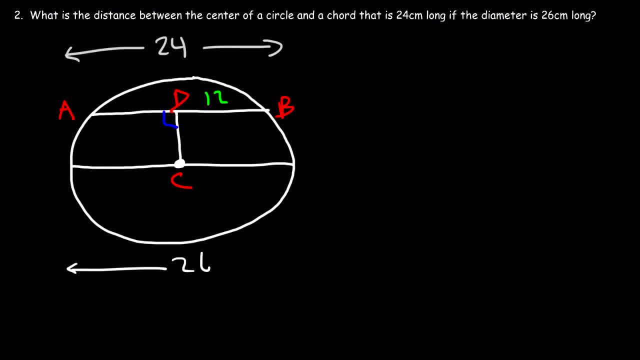 Now we're told that the diameter is 26 units long. So let's call this E and F. So C is the center. That means CE and CF. Okay, They're congruent. They're the radius of the circle. So the radius of the circle is half of the diameter. 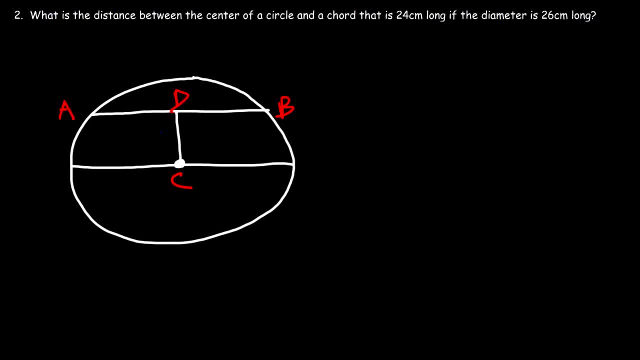 So d is the midpoint of a b, as long as c d is perpendicular to a b. Now we know that the chord is 24 centimeters long, So a b is 24.. And since c? d is perpendicular to a b, a d is equal to d b. 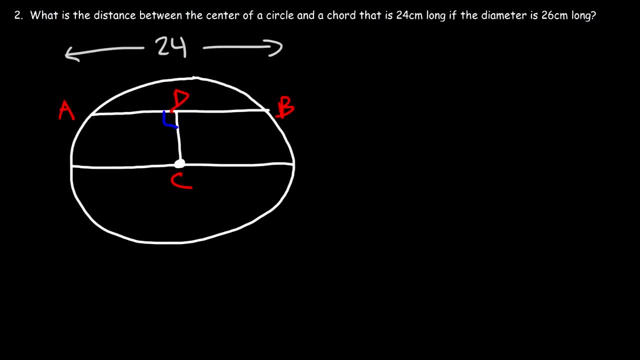 Those two segments are congruent, which means d, b has to be 12.. Now we're told that the diameter is 26 units long. So let's call this e and f. So c is the center. That means c, e and c, f. they're congruent. they're the radius of the circle. 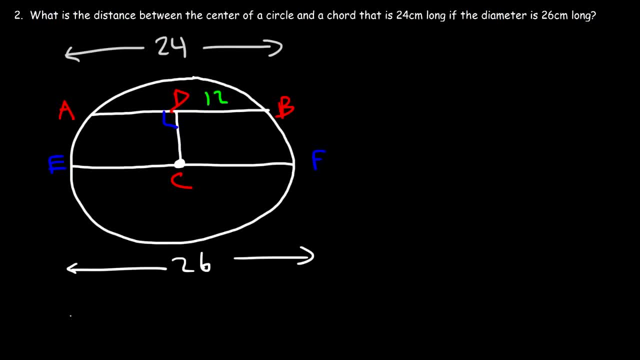 So the radius of the circle is half of the diameter, So r is one half of d, Half of 26 is 13.. So c, f is 13.. So how can we calculate x, c, d, the distance between the center of a circle and the chord? 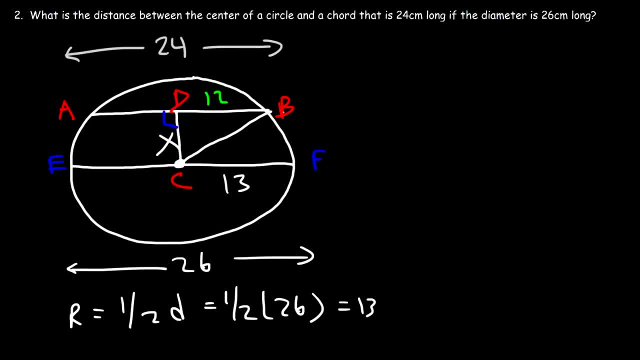 Now, If we make a right triangle, Okay, Notice that c, b is also 13.. The distance between any point on a circle and the center of the circle is the radius of the circle. So now we just got to find the missing side length of the right triangle. 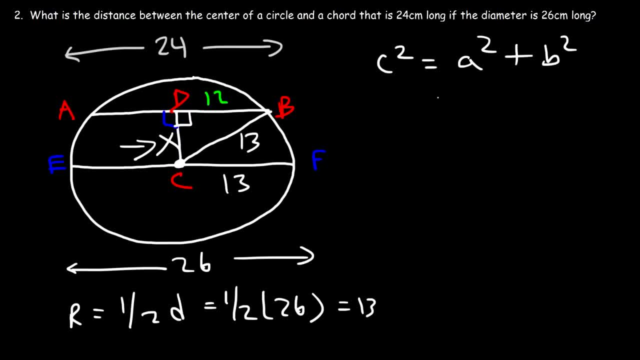 So c squared is equal to a squared plus b squared. So let's say a is x and b is 12 and c is 13.. 13 squared is 169.. 12 squared is 144.. 169 minus 144 is 25.. 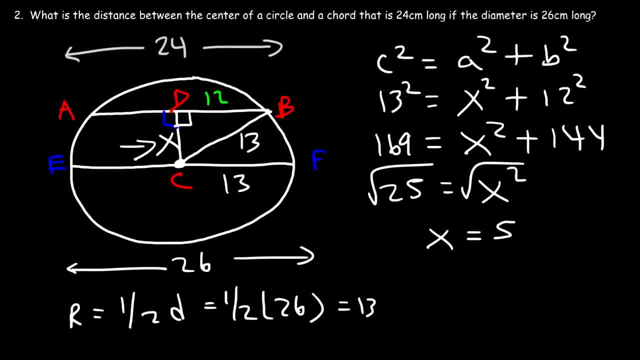 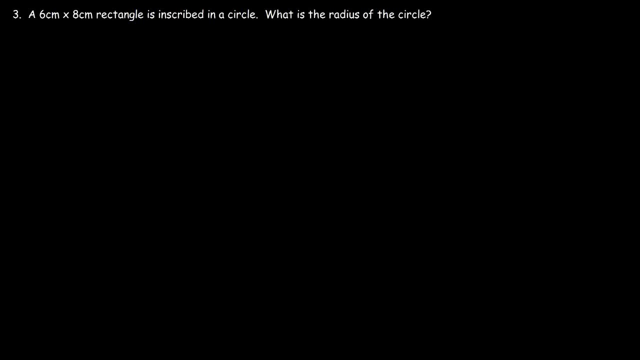 And the square root of 25 is 5.. And so that's the distance between the chord and the center of the circle. A 6 by 8 rectangle is inscribed in a circle. What is the radius of the circle? Feel free to pause the video and try it. 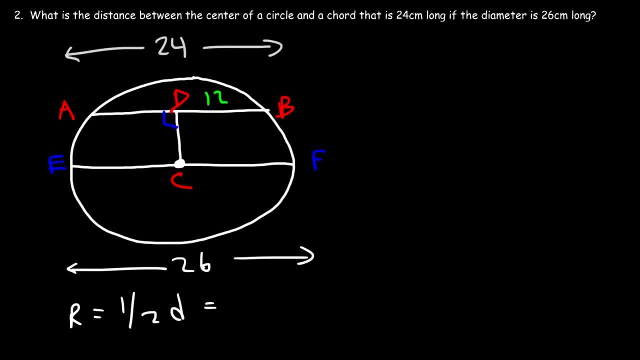 So R is one, half of D, Half of 26 is 13. So CF is 13.. So how can we calculate X, CD, the distance between the center of a circle and the chord? Now, if we make a right triangle, 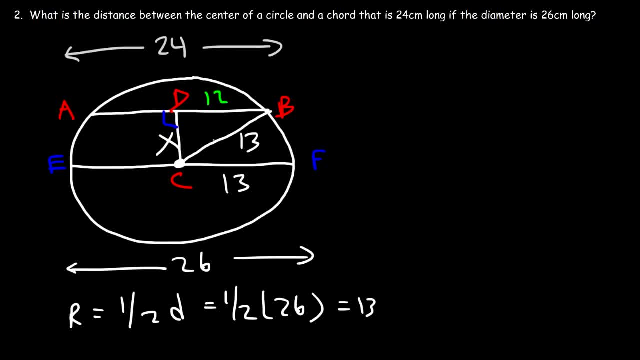 Notice that CB is on the right. It's also 13.. The distance between any point on a circle and the center of the circle is the radius of the circle. So now we just got to find the missing side length of the right triangle. 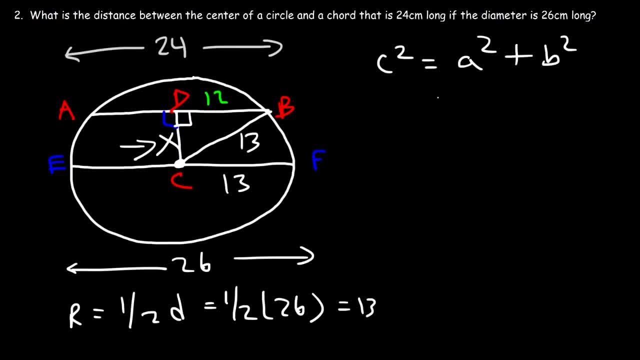 So C squared is equal to A squared plus B squared. So let's say A is X and B is 12 and C is 13.. 13 squared is 169.. 12 squared is 144.. 169.. 169 minus 144 is 25.. 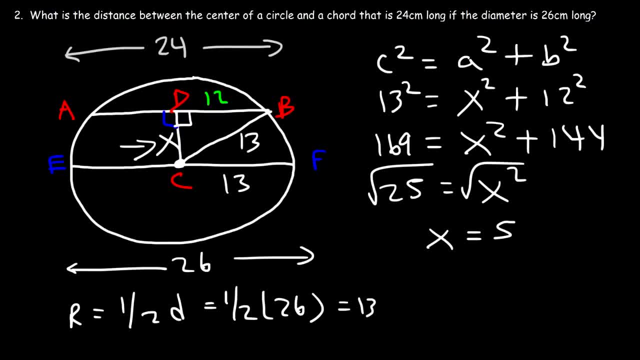 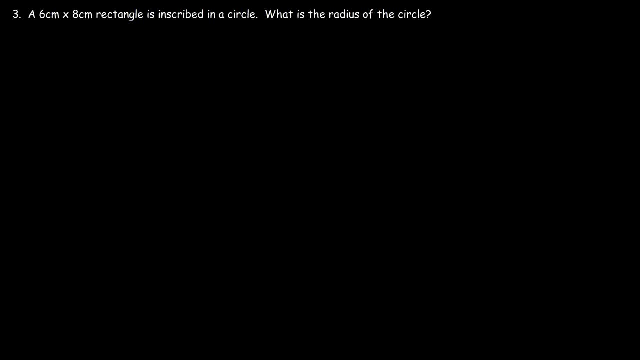 And the square root of 25 is 5.. And so that's the distance between the chord and the center of the circle. A 6 by 8 rectangle is inscribed in a circle. What is the radius of the circle? Feel free to pause the video and try it. 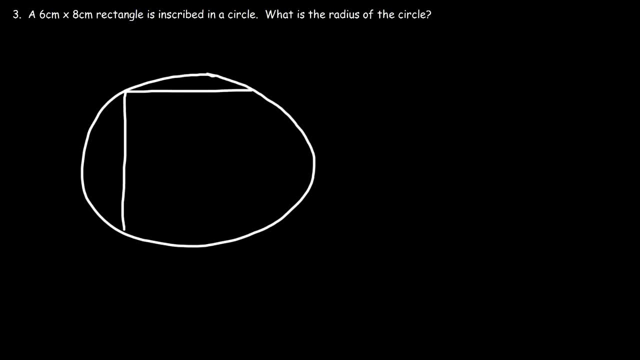 So the rectangle is inside of the circle And let's say this is the center of the circle. Now let's call this AB and DF Or DE, And this is going to be center C. So the radius is from the center to any point on the circle. 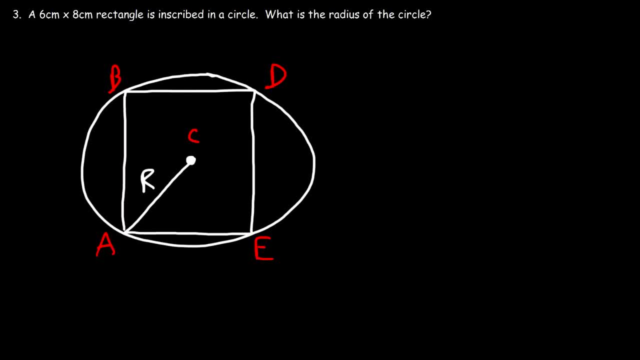 So we can say that AC represents the radius. Now AE that's going to be 6 centimeters long, And DE, that's 8 centimeters long. So if we draw a point, let's say the midpoint of AE. let's call that point F. 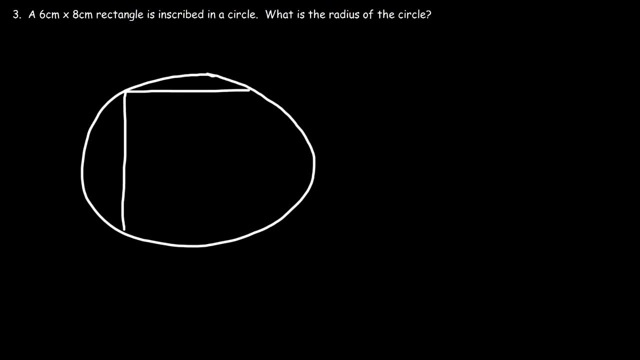 So the rectangle is inside of the circle And let's say this is the center of the circle. Now let's call this a, b and d f or d e, and this is going to be center c. So the radius is from the center to any point on the circle. 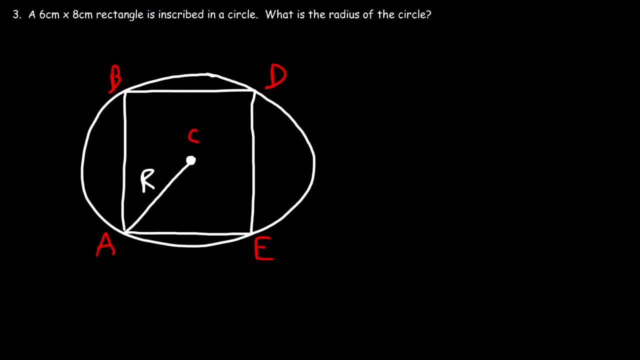 So we can say that a- c represents the radius. Now a- e- that's going to be 6 centimeters long, And d- e, that's 8 centimeters long. So if we draw a point, let's say the midpoint of a- e. 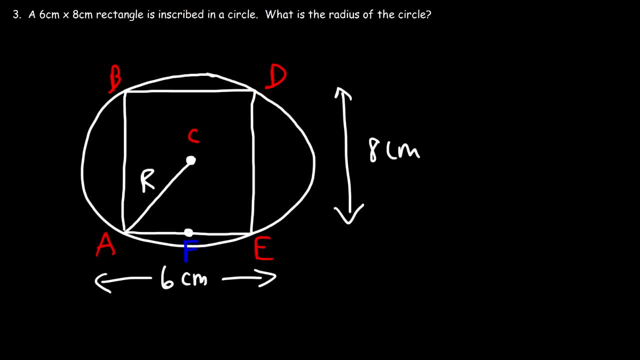 Let's call that point f. Then a f has to be half of a? e, So a f is straight. c f has to be half of d? e, So that's going to be 4. Because the center is basically the midpoint between the diameter of a circle. 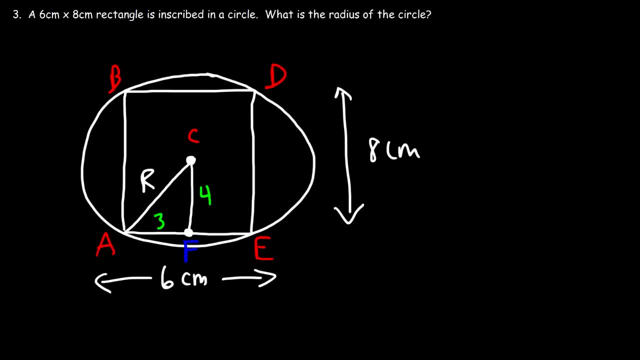 It's like in the middle of the circle. So c f has to be half of d, e, a f has to be half of a, e. So now we can calculate the radius. So c squared is equal to a squared plus b squared. 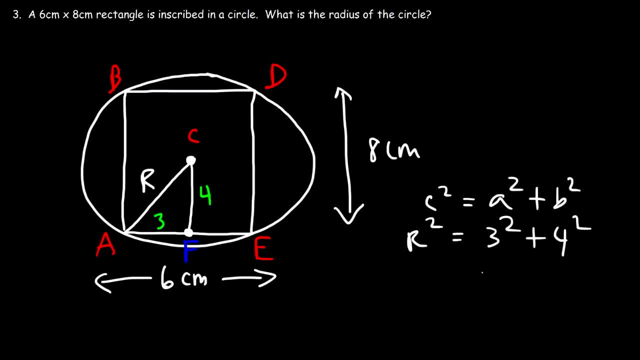 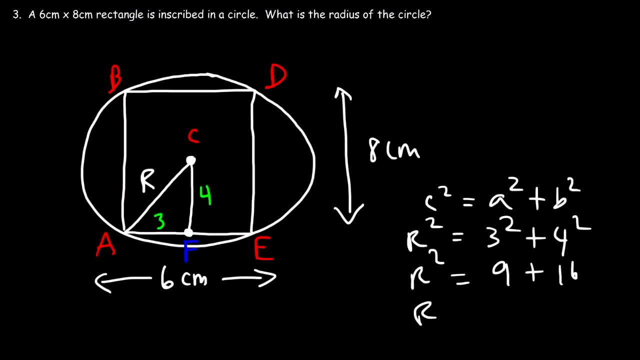 3 times 3 is 9.. 4 squared is 16.. And 9 plus 16 is 25.. And the square root of 25 is 5.. So that's how you can calculate the radius of a circle. if you have a rectangle, that is. 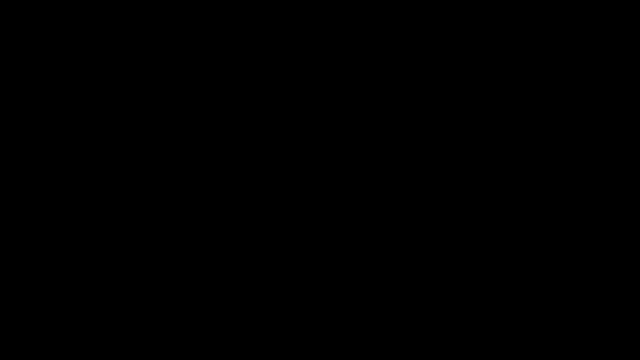 inscribed inside of a circle. So that's how you can calculate the radius of a circle.